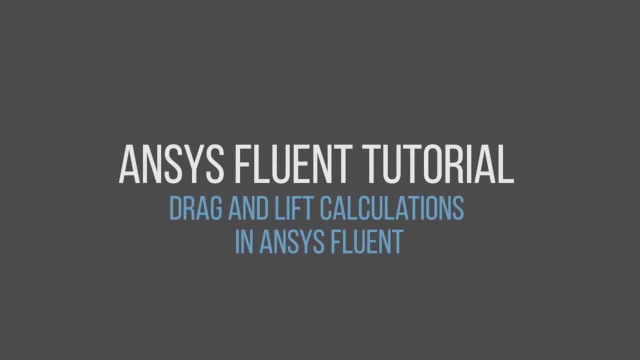 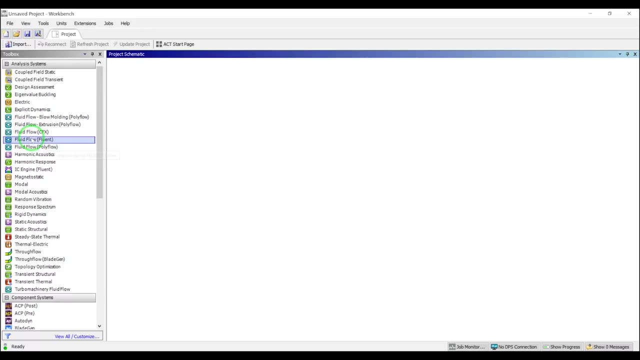 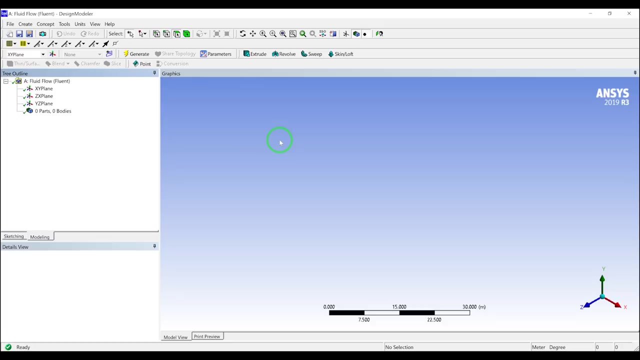 Hello everyone. in this video I'm going to show you how to calculate a lift and drag coefficients- a lift force and drag coefficients in ANSYS Fluent. First I'm going to use Design Modeler to create a geometry, something like a truck- commercial trucks. Then, based on that, I will 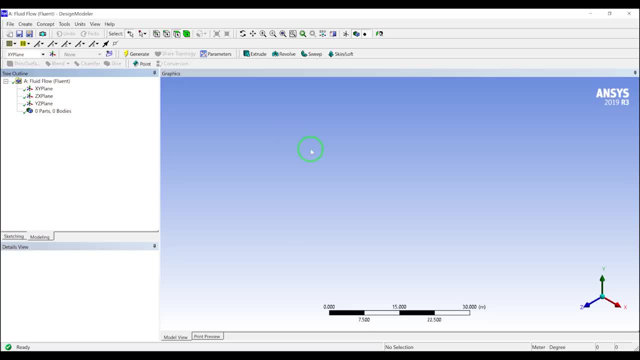 calculate the drag forces and drag coefficient and lift forces. So here I will go to XY plane. create a new sketch and I will keep the units as meters. So here I will go to Sketching. I will zoom in a little bit, so I will create a Rectangular. 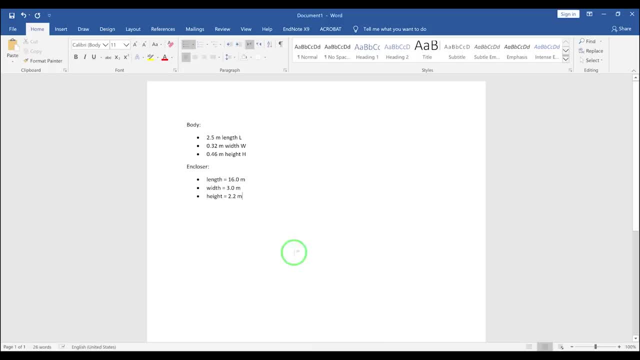 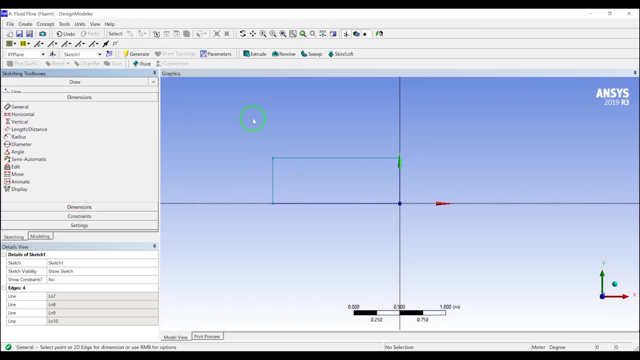 Okay, so the body I'm going to create is 2.5 meters in length, 0.32 in width and 0.46 in height, So I will use the dimensions general let's define as 2.5, and for the height I have 0.46.. 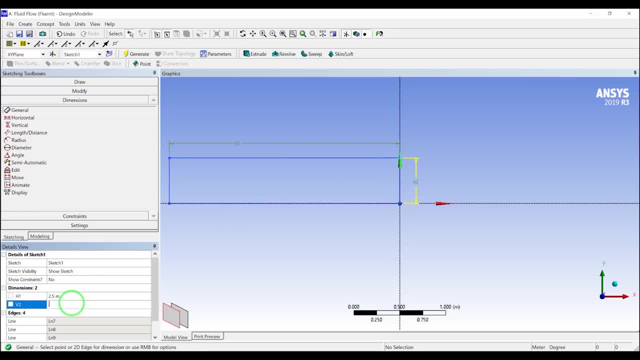 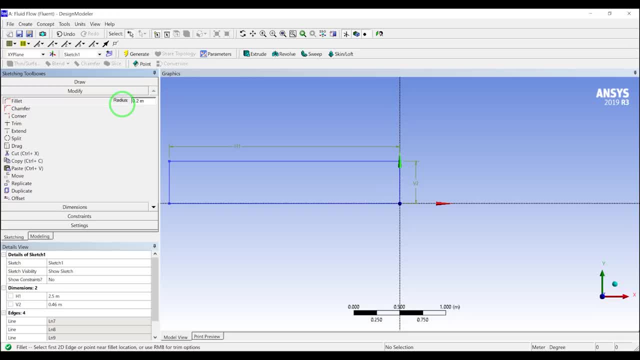 I will create a fillet. So the radius should be lower. let's try 0.2.. Okay, so I will create some a little bit aerodynamic shape in the front. So I will go to Modeling, Sketch, Extrude, Sketch, Direction. I will do the symmetric direction. so 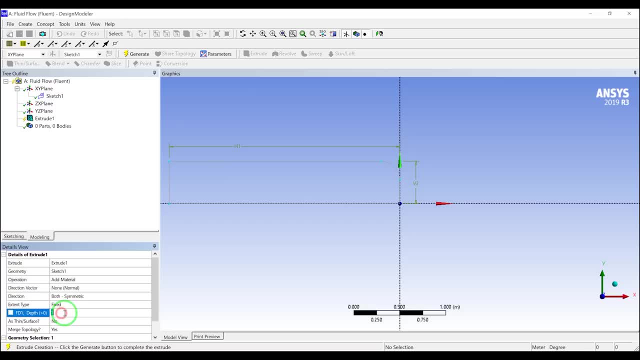 each side will be point 16. so I will put point 16 here. so it will go point 16 to each side. so I will press generate. now we have our truck body. the next step is to click and create an enclosure. so I will as a airfield, so I will create an. 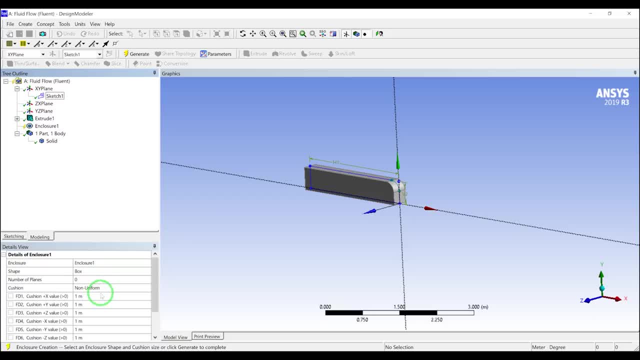 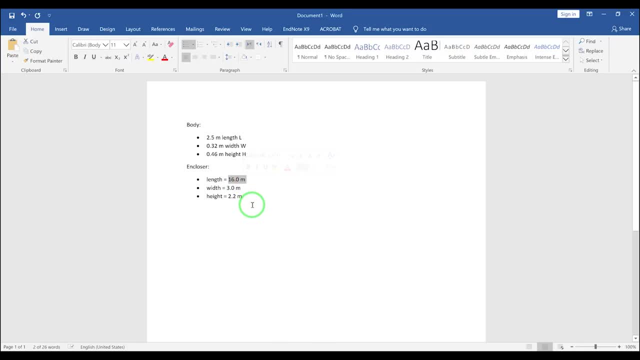 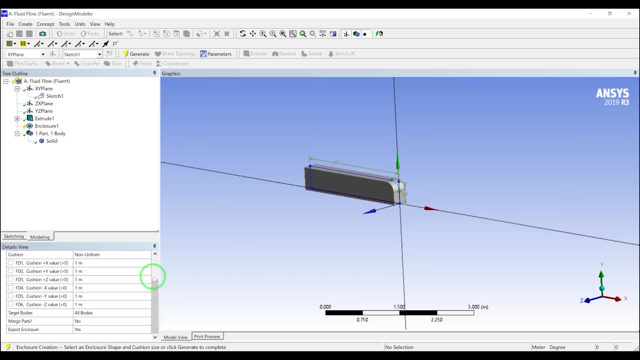 enclosure. so for the enclosure, I will use point 16 meters in length, which means: which means that 8 meters and 16 meters in length, which means 8 meters in each side. so in X Direction I will put 8 and in minus X Direction I will put 8. for. 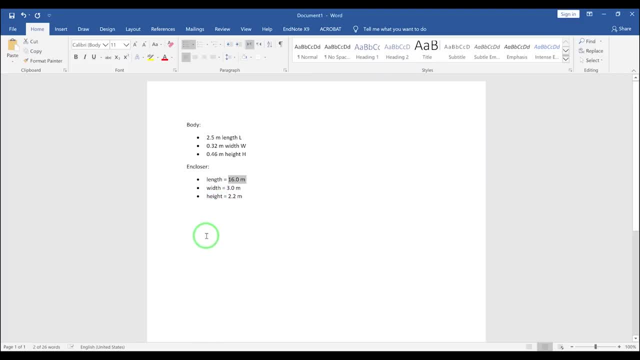 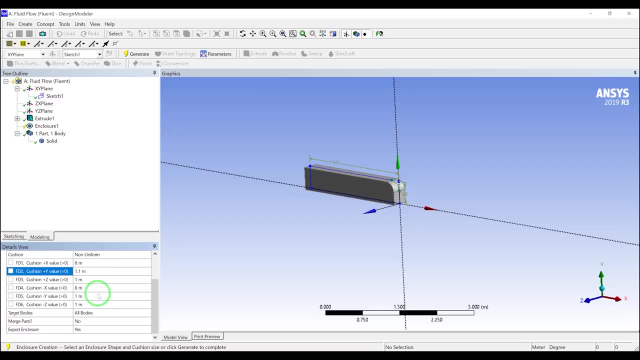 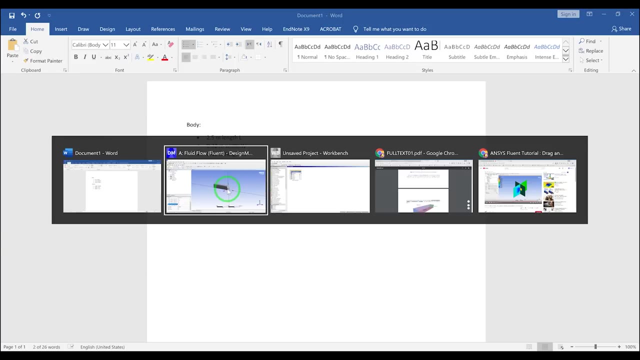 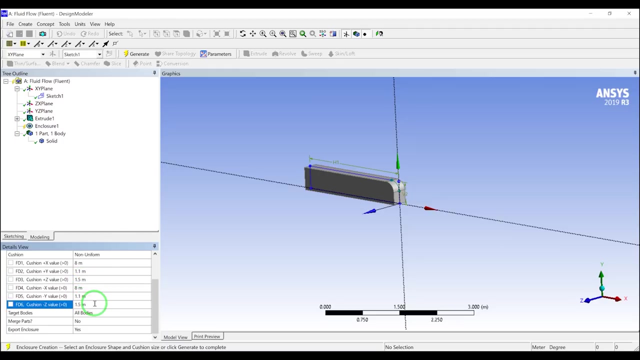 height is 2.2 means that's 1.1 in each direction, 1.1. 1.1 then, and in the width 1.5, which means in the Z direction, 1.5, here, 1.5 here. so I will press generate. so this is the enclosure, or something like a wind. 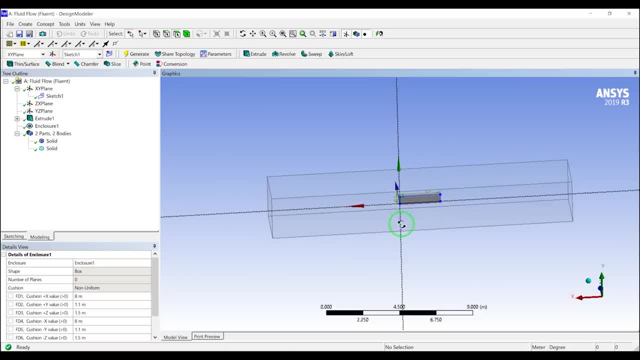 tunnel. we are going to test on this like almost truck shaped body. so here we can go to full and to meshing and fluent use both of these bodies. but since we don't need the body of the truck, we don't want to calculate the heat transfer. 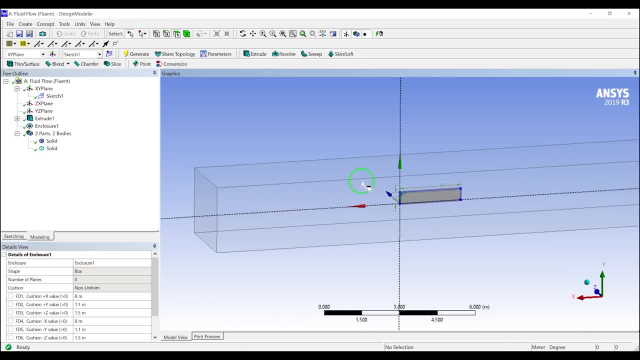 coefficient. so I will go and subtract this truck body from the air. so, because I only need the shape of the truck in the air. so I will go and subtract this truck body from the air. so, because I only need the shape of the truck in the air. 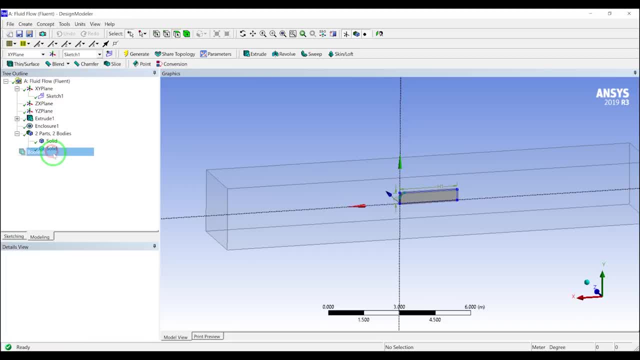 so I will go and create a boolean and subtract. so the target body, this one tool body, is truck and I don't need to keep the tool body or truck, so I will subtract this one, so I will have one body as the air. so I will close the design model. 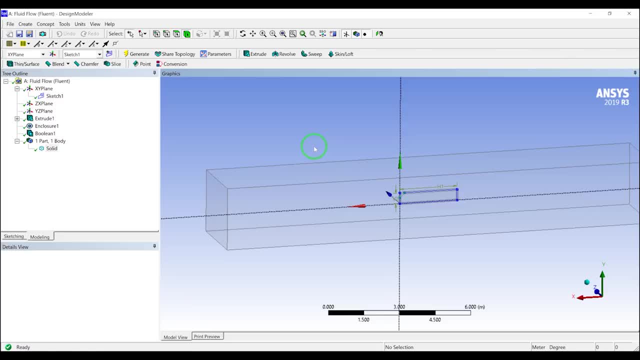 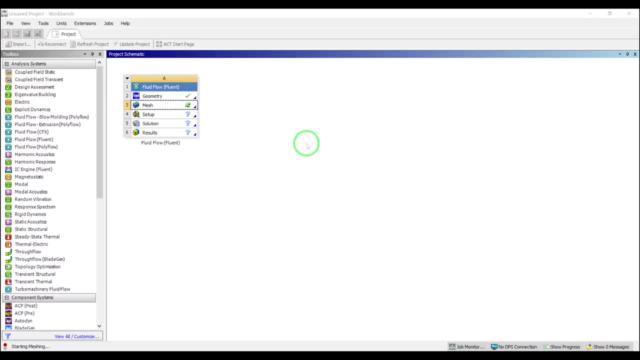 as the air. so I will close the design model as the air. so I will close the design model there and open the machine. so I will there and open the machine. so I will there and open the machine. so I will go ahead and open the machine. go ahead and open the machine. 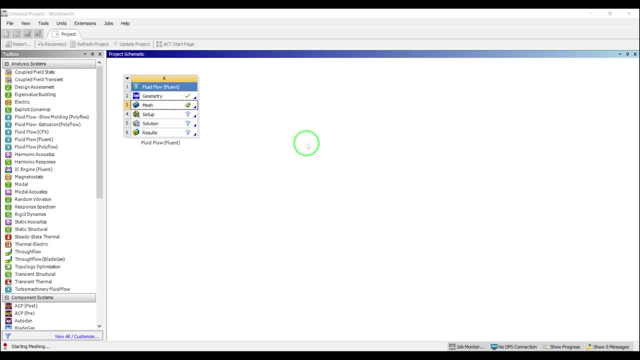 go ahead and open the machine. so in this tutorial I'm using the ansys. so in this tutorial I'm using the ansys. so in this tutorial I'm using the ansys machine, but in the newer versions that machine. but in the newer versions that machine, but in the newer versions that fluent machine is very powerful and it. 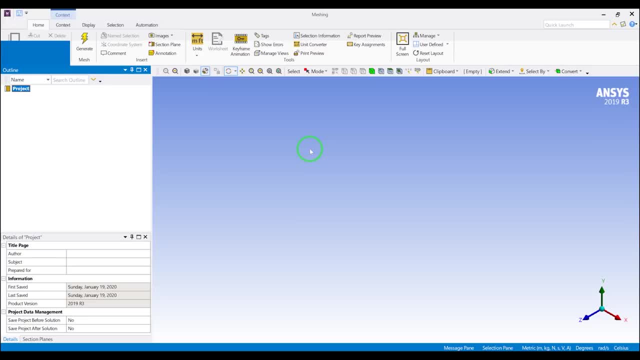 fluent machine is very powerful and it fluent machine is very powerful and it has very nice tools, so I will try to has very nice tools, so I will try to has very nice tools, so I will try to post some videos about the post, some videos about the. 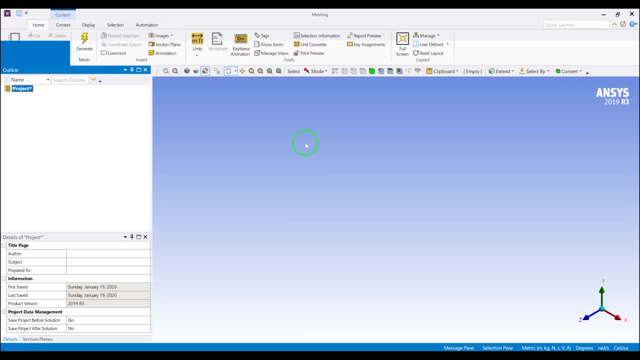 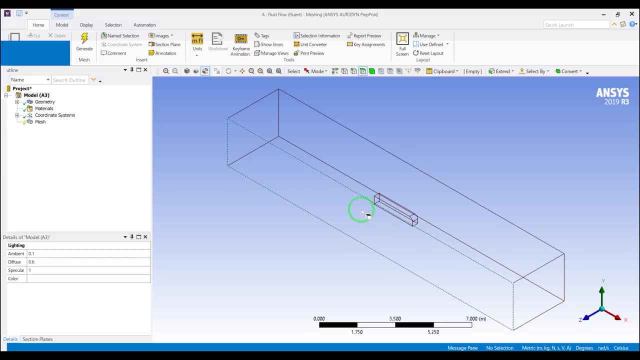 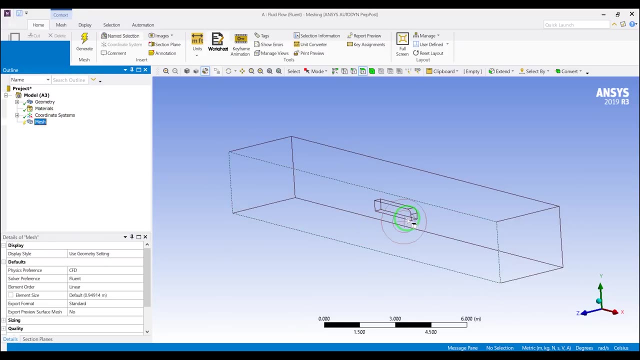 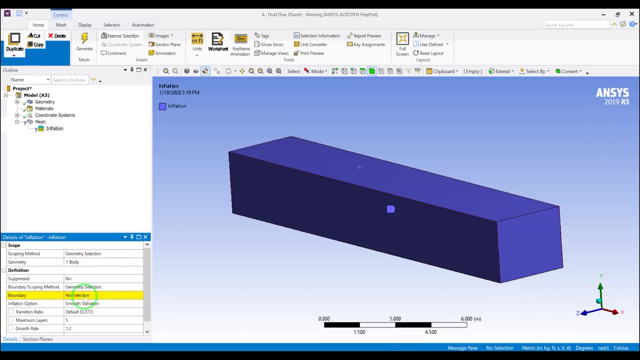 how to use the fluent meshing and you will see how effective and easy you can is the fluent meshing these days in the newer version. so here I will create some inflations or boundary mesh layers on this truck body. so I will go and insert, I will select inflation, so the geometry, I will select the body as this one and for 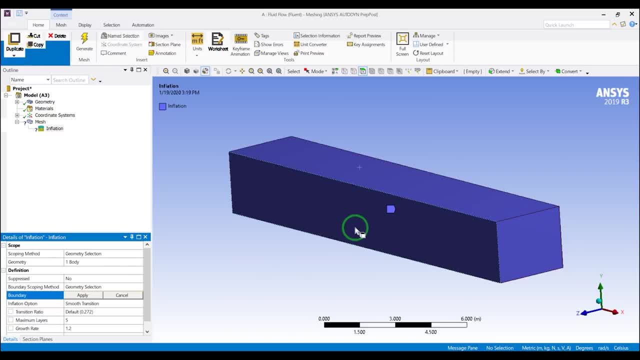 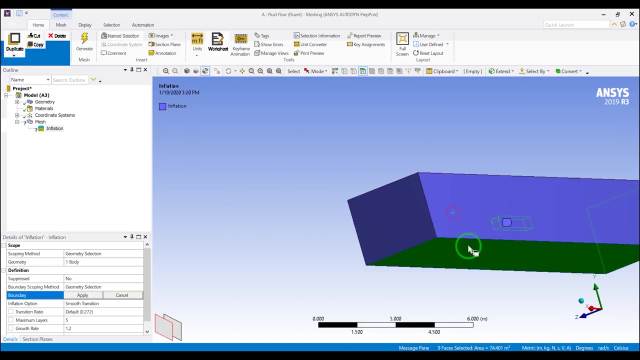 the boundary. I need to select the whole truck bodies. I will select press ctrl, enter a, so it will select all of the surfaces and, like holding down the control, I will deselect the enclosures, outer walls, or so I deselect all of these six bodies and I have to selected this truck body wall. so I will go ahead and apply. 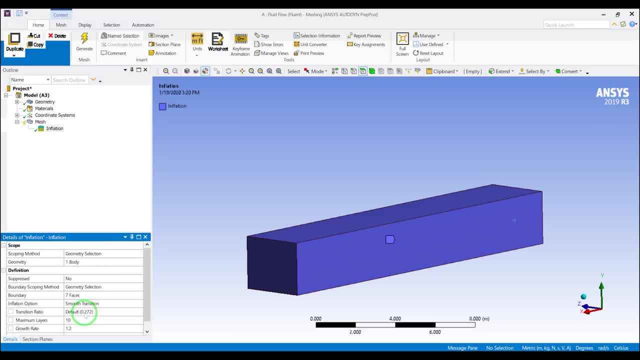 so I want to have a ten layers of inflation layers around it, try to capture as much as I can the vorticity turbulences, and then I will go for the sizing. I want to have the maximum size of half a meter because, and so this one should be smaller than that 1.2 for the element size I will generate. 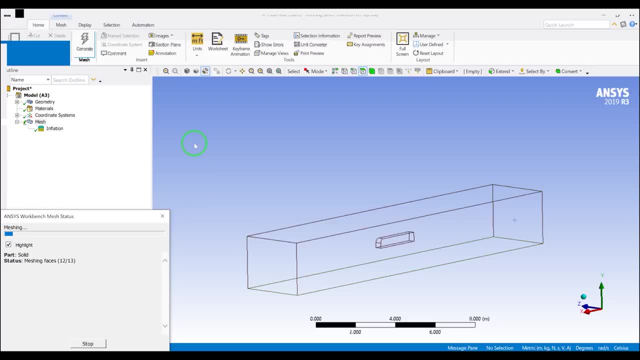 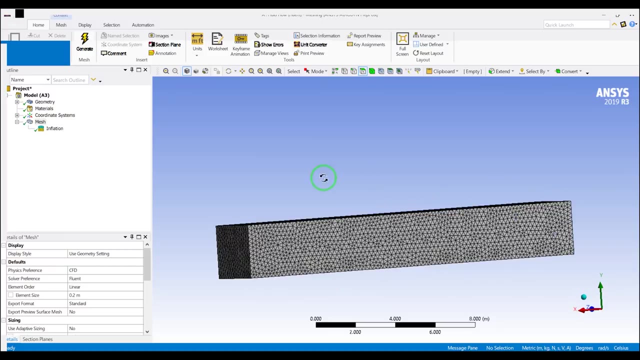 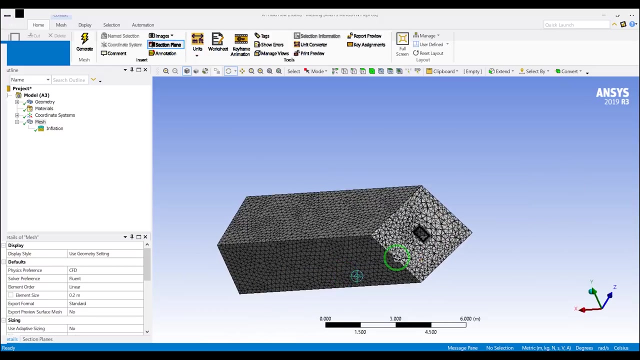 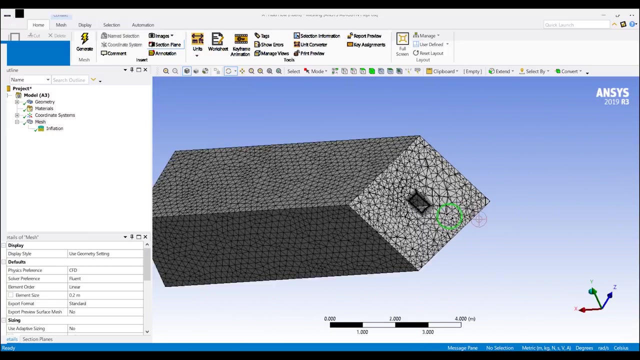 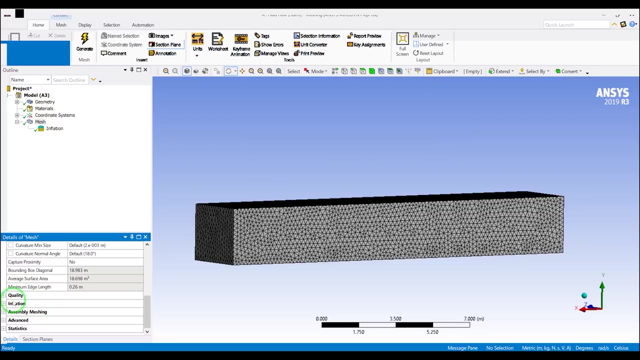 the mesh to see what it looks like. okay, we have our mesh here. let's create a section plane. cut through the mesh to see how it looks like. you can see that it has nice layers around the truck body and we have a mesh, so I will select this one and I want to see the quality. I want to see how is the skewness? 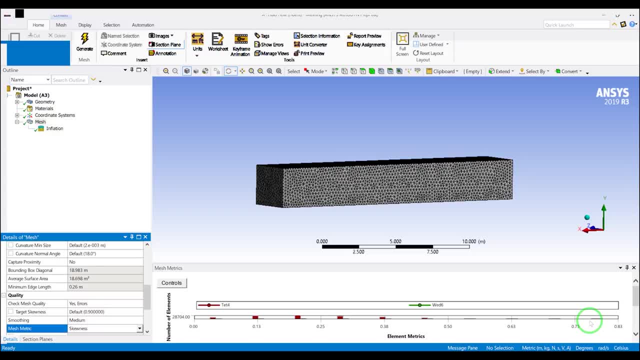 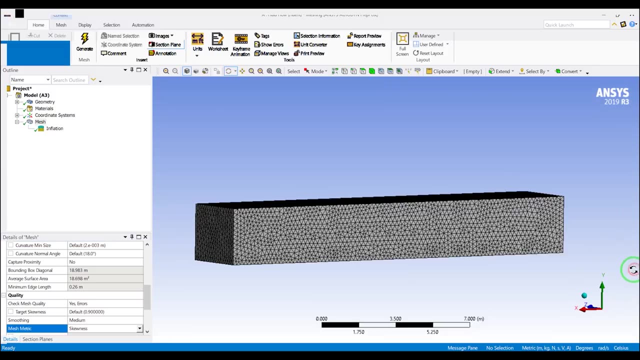 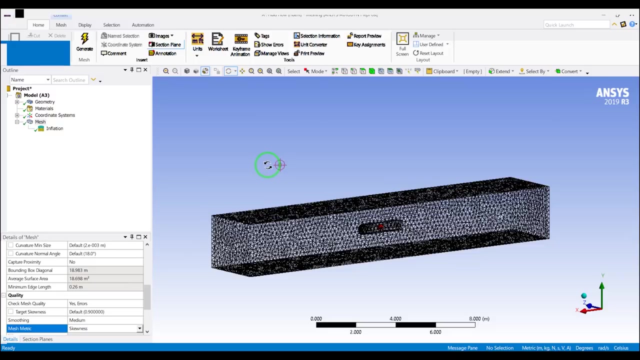 so the skewness is less than 0.83, so it looks okay to me for this calculation. it should be as low as possible, for for this calculation it's okay. so it's also common to check the orthogonal quality. but um, I will convert the mesh in fluent so we don't need to worry about that one, so front. 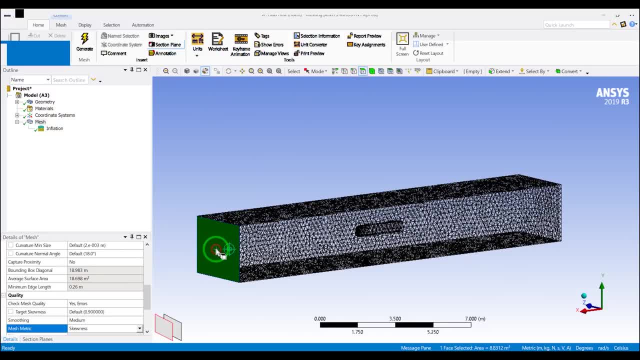 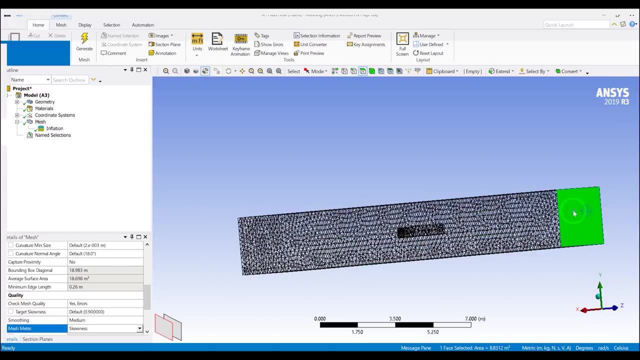 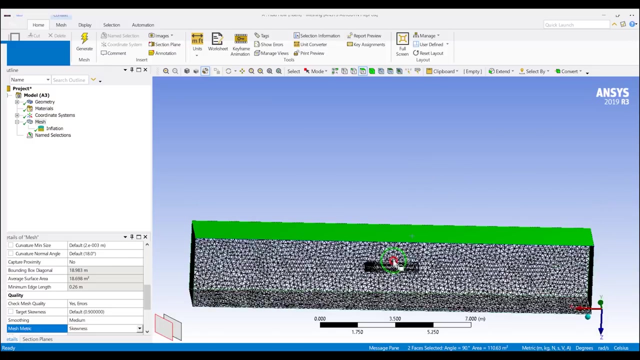 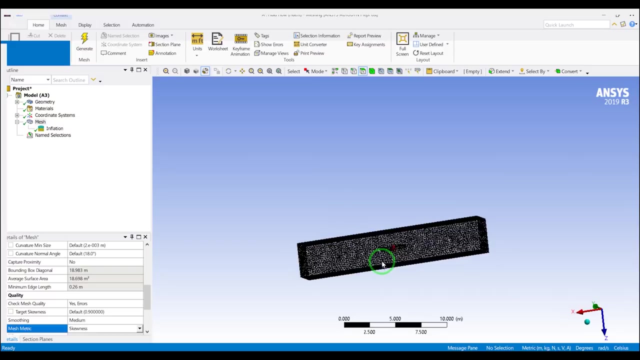 side of the truck is the inlet, so I will define this one as name selection. the shortcut is n, so inlet, and I will define this side as outlet. press n outlet. so I will select these, define as walls, and also I will select all, deselect these to define a name selection for the truck: body. press n and name it truck. then I will go ahead. 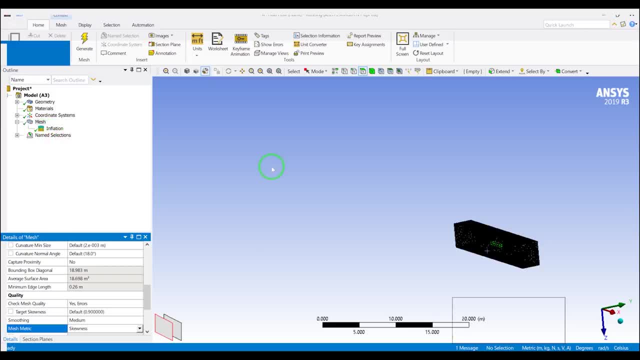 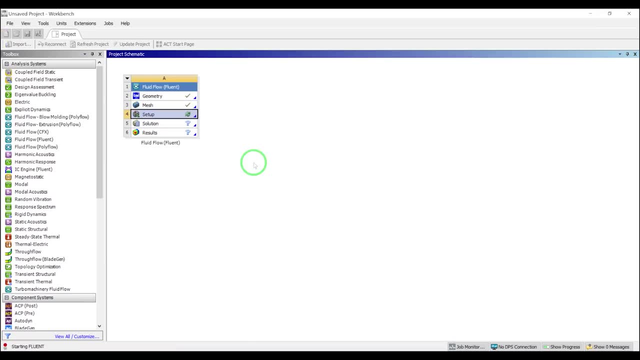 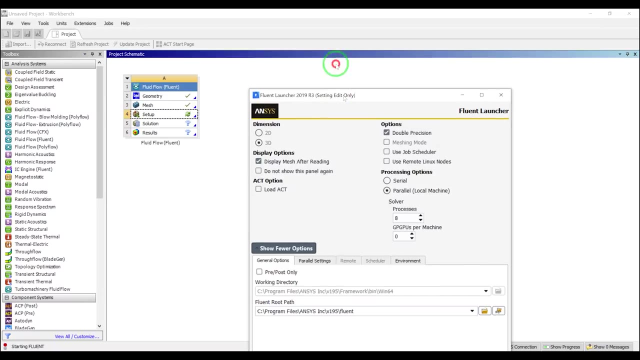 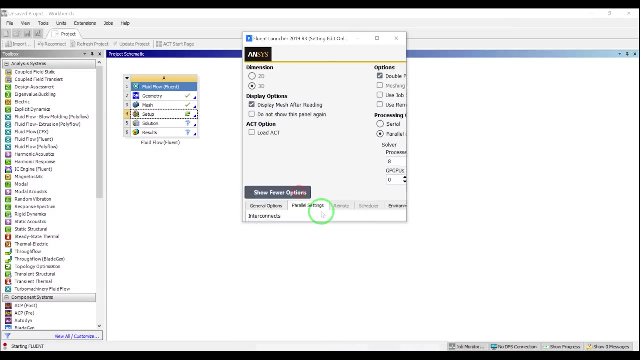 and update the mesh. so it will send the mesh to the fluent, so I will minimize this meshing open fluent, so I will use parallel. I have eight CPUs. I'm using the Intel CPUs and I have installed the Intel MPI on this machine, so I will select this one. 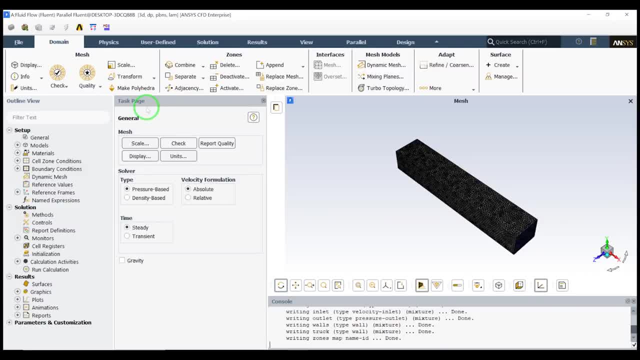 now we have the fluent open, so the first thing I will do is convert our mesh to polyhedra, which has a better convergence quality and faster influence. so okay, it's done and suggest to reorder our partitions as in the parallel solving after converting the mesh. so I will run these. 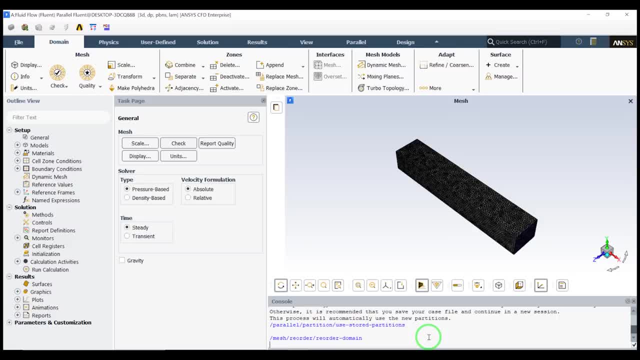 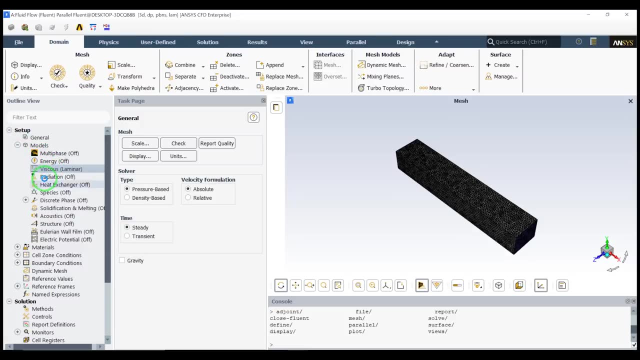 commands. okay, it's done, so I will mainframe it with these two other parts mit quantity of Abigail. so this is probably the most accurate one because of the overall configuration of this particular model. so on out which one we are going to use and candidates that are available in this instance, are created, the ones that are already configured for us. so let's see which one we want to run. Fred, when it comes to subnets, what the test costs and so over, see what's present here. it fits perfectly. so we are going to check if it's boxed on top of the fluid that's real and used, the sstk omega turbulence model and material. we need only air. so I will have, for this cell zone, which is the Floyd, we have one single sell zone. 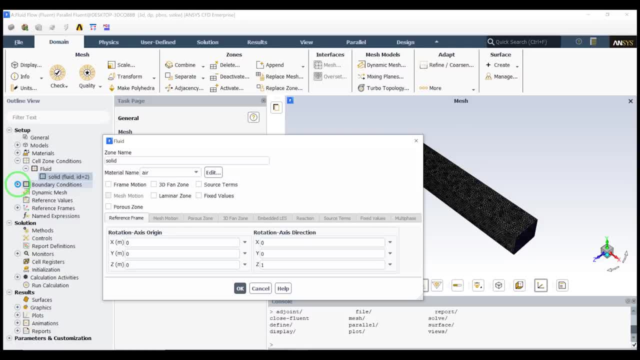 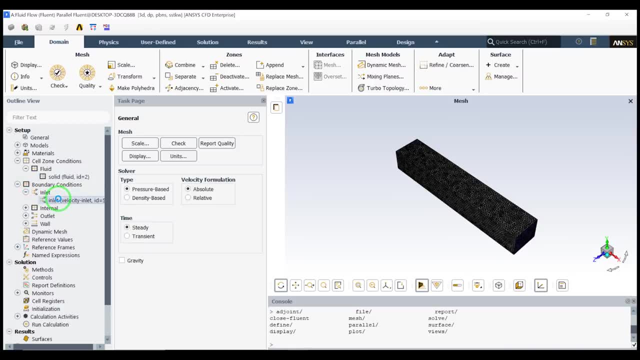 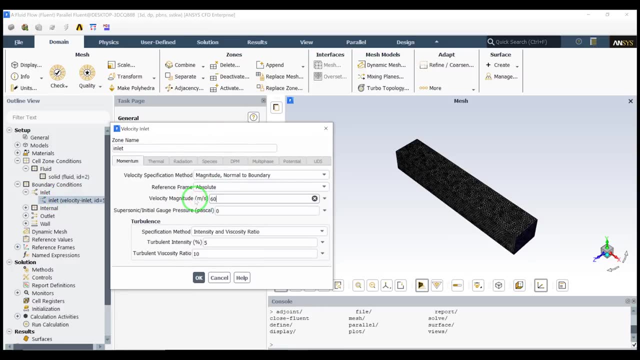 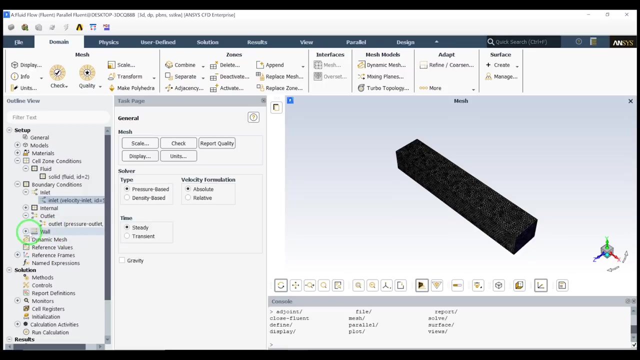 is. so for the inlet, i will define the 60 meter per second of the airflow from the inlet and i will leave the outlet as a pressure outlet and i will not touch the walls. so i will go ahead and close this boundary condition. so for the, and to calculate the drag. 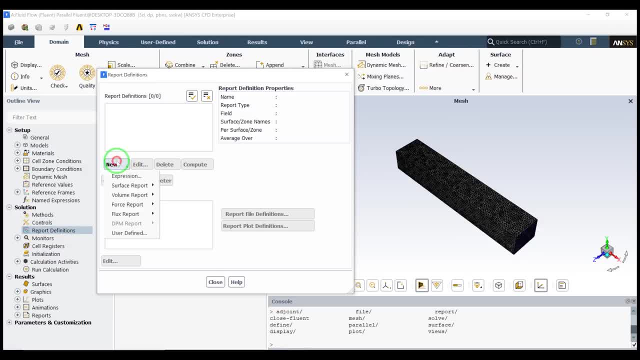 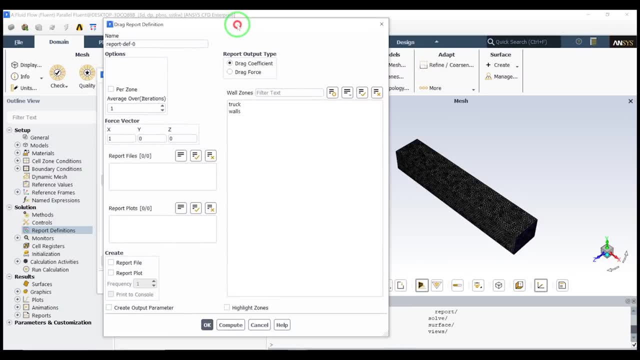 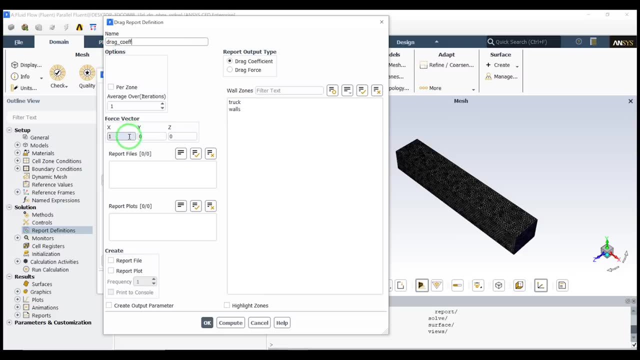 coefficient, we will go to the report definition. new force report: drag. so in this window i will name this one as drag coefficient. so the m, this is the fact. force vector in this window. so this is the force vector in this window. so this is the force vector in this window. 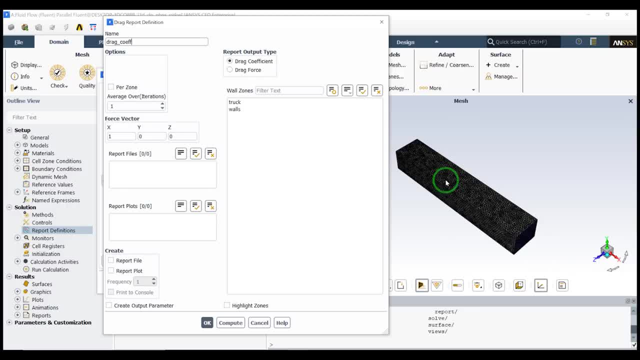 which direction you want to calculate the drag force. in our case this is in the x direction because we have the airflow in the x direction. so i will keep this one as one, zero, zero. so i want to report to a file and plot this one. the surface i want to calculate is the truck as i selected. 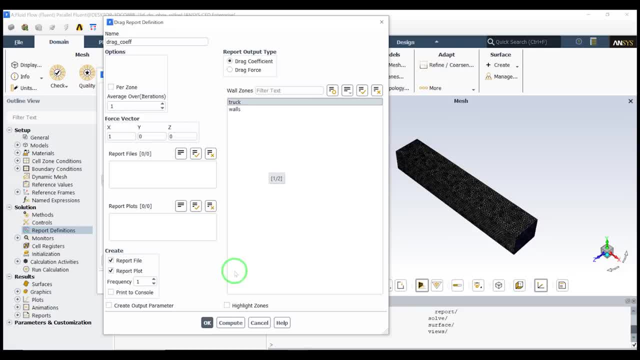 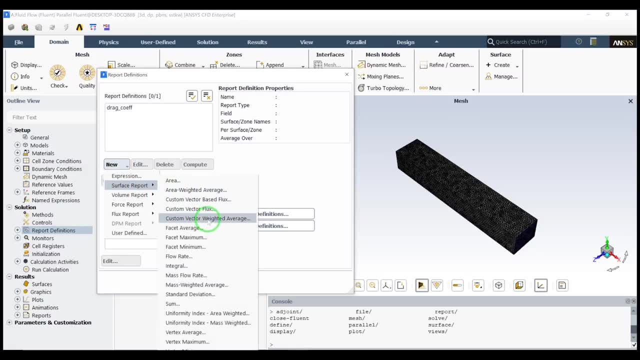 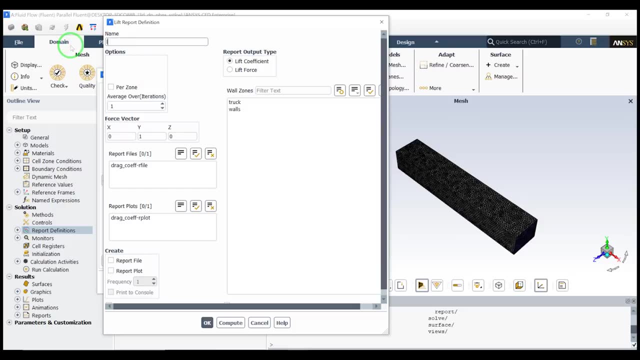 and defined the name selection in the meshing, so i will click ok. also, we need to calculate the, the lift force, to see what's the lift force. so i will go to lift force. so this is the lift coefficient on truck and the direction is y. so because lift is in the y, 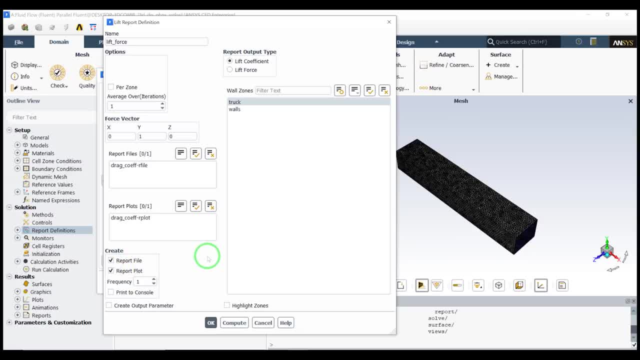 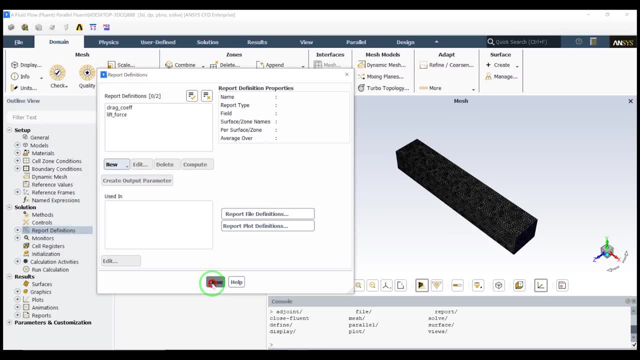 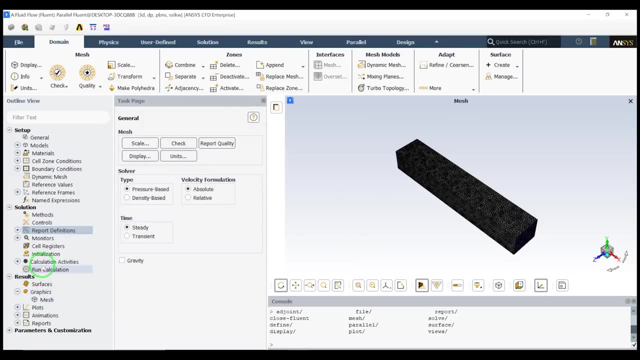 direction for this case. so i will. i want to report to the file and plot and press ok. so we are done with the, with the, our reports. so also i want to. i will run first, then do the counters, so i will initialize and personalize the results, ok. 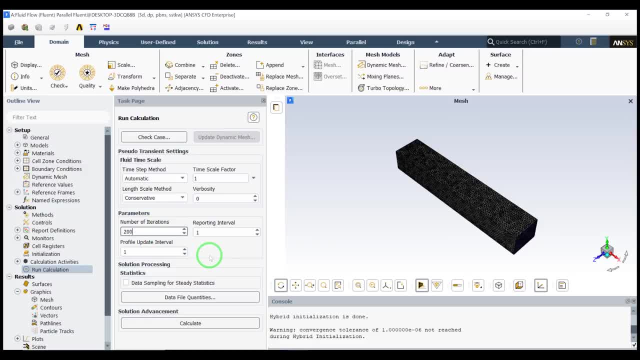 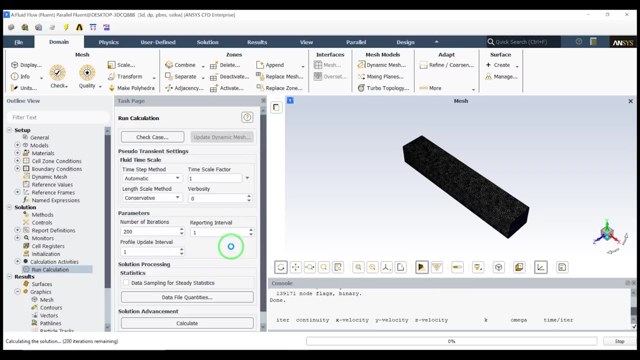 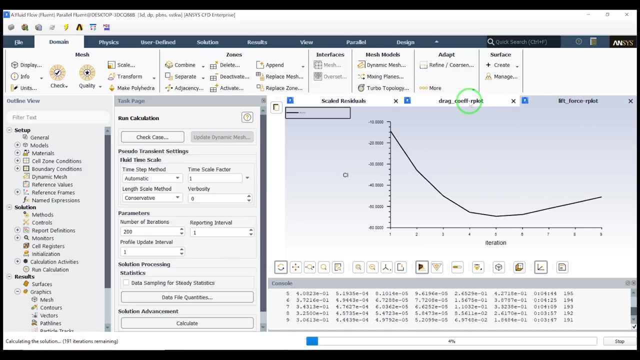 i want to do the 200 time steps, or 200 iterations, to see if it will reach the convergence. so, as it solves the problem, it will calculate the lift and drag force coefficients in each iteration. so I will pause the video and when it's converged I will continue. so now our solution is converged. 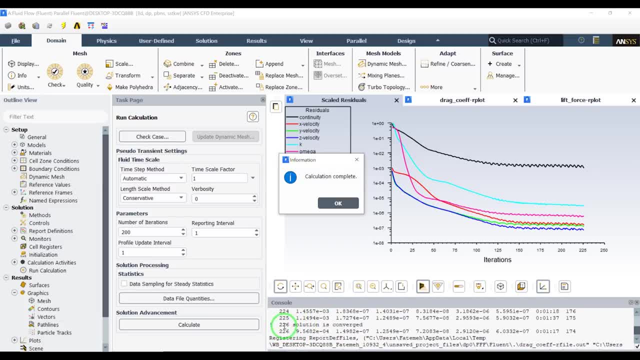 and we didn't converge at 200 times iterations, so I am pressed to calculate again in 226 and the solution was converged. so I will go ahead and, as you can see, we have a and and error in the drag coefficient at the beginning then, but it kind of converged to a constant number. 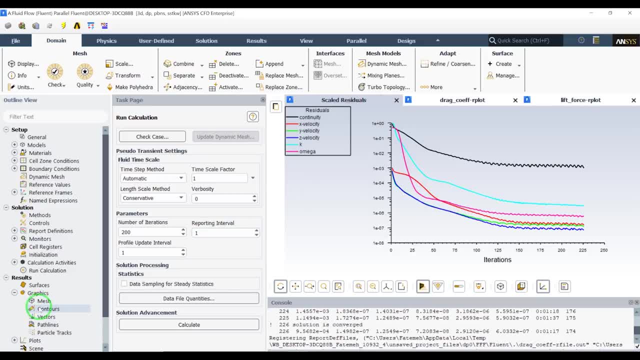 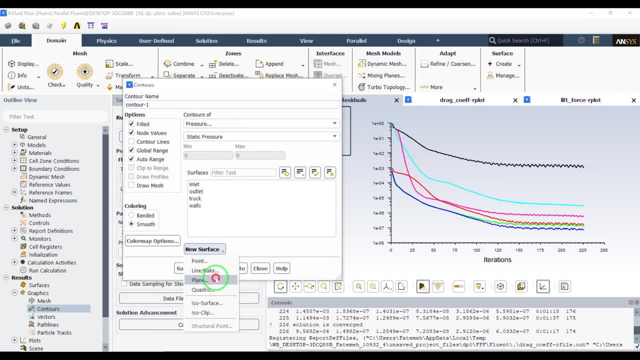 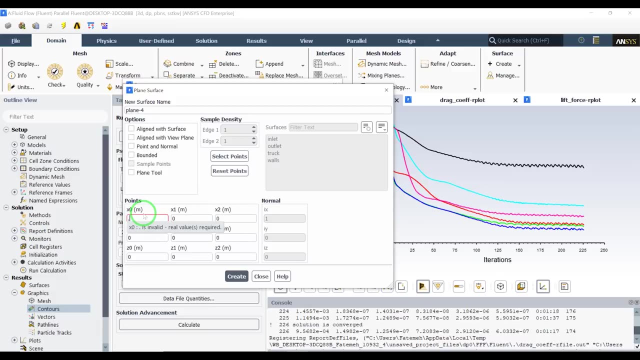 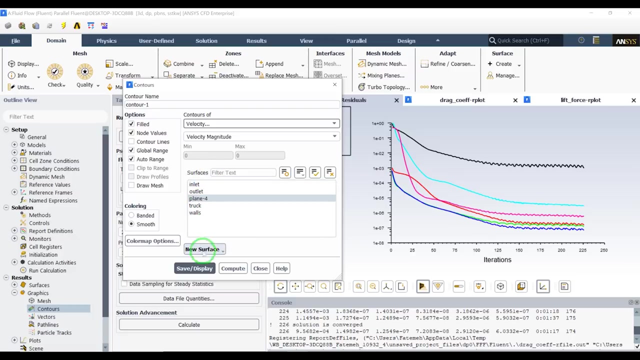 so let's plot the velocity. so I will define a plane in x- y and x- y plane, so I can put any arbitrary number here and just put the z's as zero and we will just plot the velocity by taking 1.. and I'll create this plane number 4, the plane number 4. I want to plot the velocity magnitude. 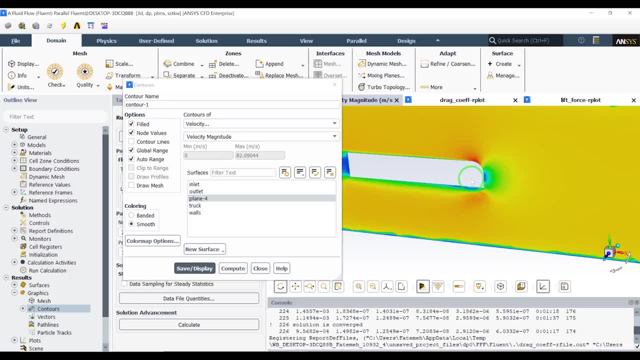 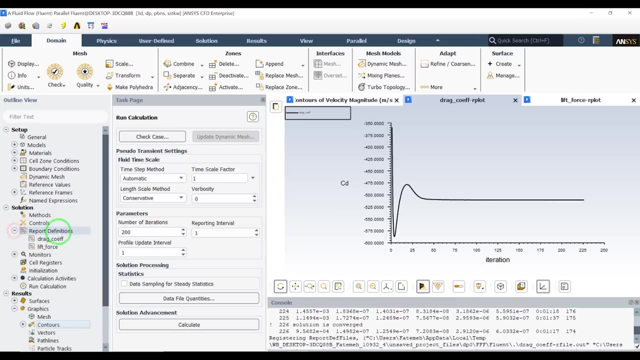 so here you can see in the X direction and this is the back of the truck. you have separation here and very low amount of drift on this plane. just a slight 무대 effect on this plane. so you also have some indicated velocity. so you have drag coefficient. if you want to see what's the drag. 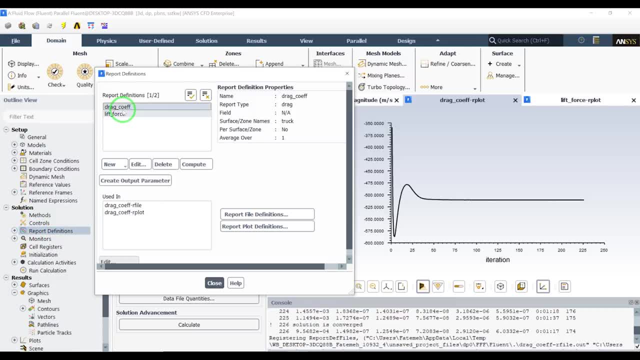 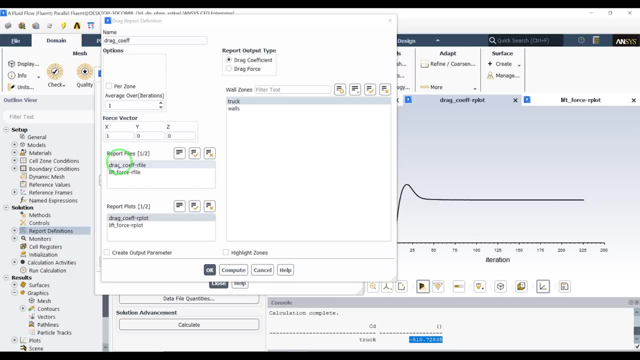 coefficient. just double click on this one and like edit the drag coefficient. press compute. you will see the amount of the drag coefficient. this is a minus value because negative value because the direction is the in opposite direction of the X direction. so we can define as a minus 1 and compute again so it will. 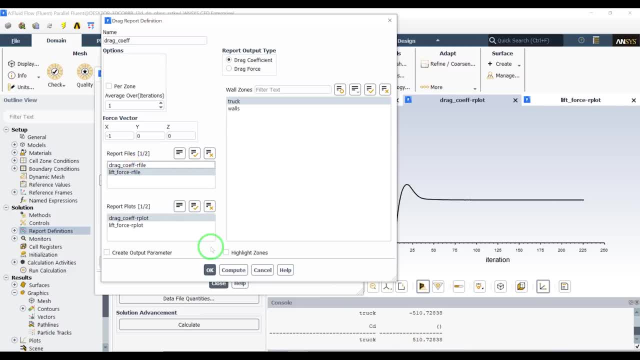 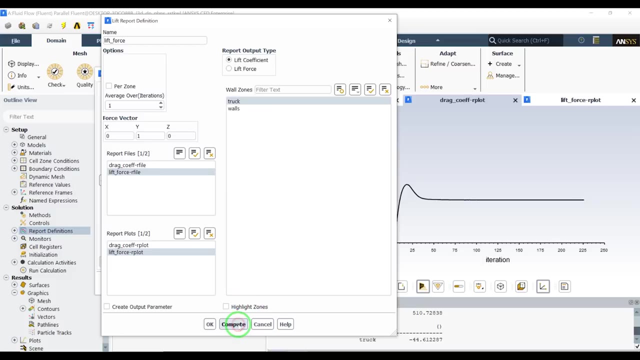 give us the positive value so we can calculate the lift force. so I will close this one- lift force, edit and compute so we have the lift force. again we can. it means that there's a press down instead of lift. so I will close this one and pause the video and open the post-processing. 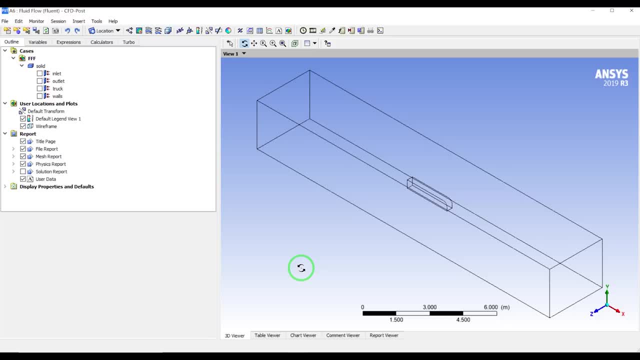 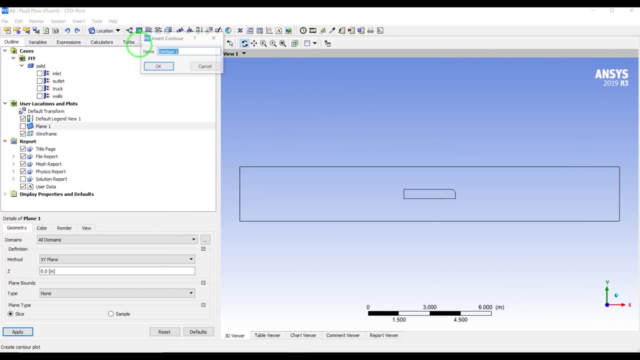 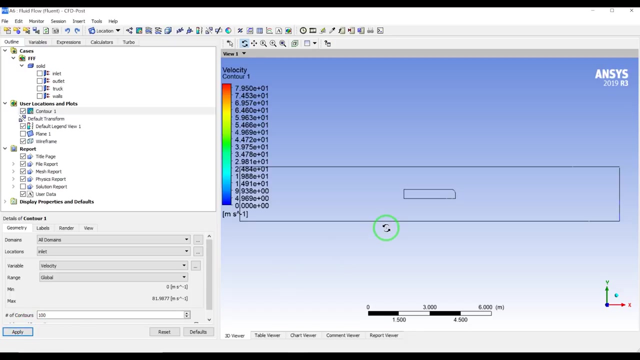 now I have closed the fluent and open the post-processing, and in the post-processing I'm going to create a plane XY, plane Y. so I'm gonna hide this plane, use that plane just as a location. so I will create a counter and let's do the counter of velocity: 100, number of the counters fly, the location is plane. 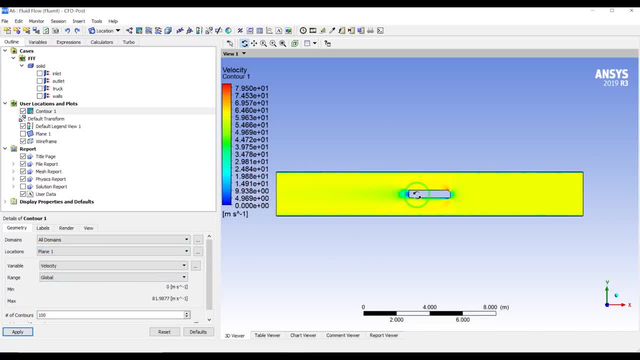 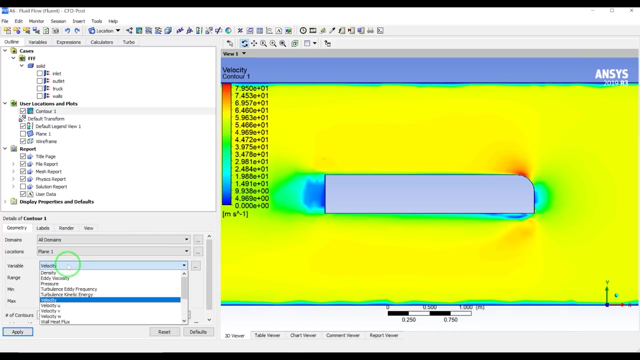 one. so and you can see that we have the low velocity stagnation point at the front and also very low velocity when let's manually match the plane. that being at the location level, the point to placement is a archetype 50 at the field, at the back, because of the separation. also, we can check the pressure. so let's see local.